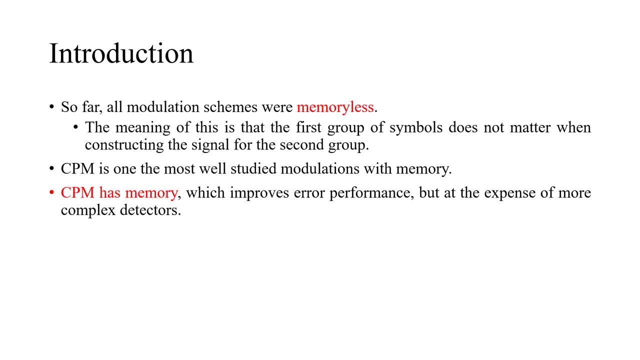 will depend on the state of the carrier for the previous symbol. That means the system is exhibiting some kind of memory. Only if you know the previous state you can decode the current symbol. So such a system will improve the error performance in total, but it will in turn increase the complexity of the system. 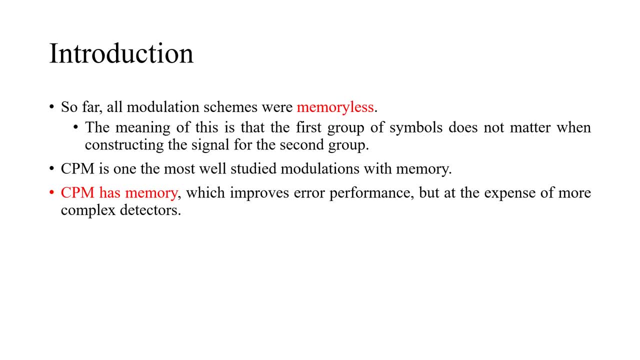 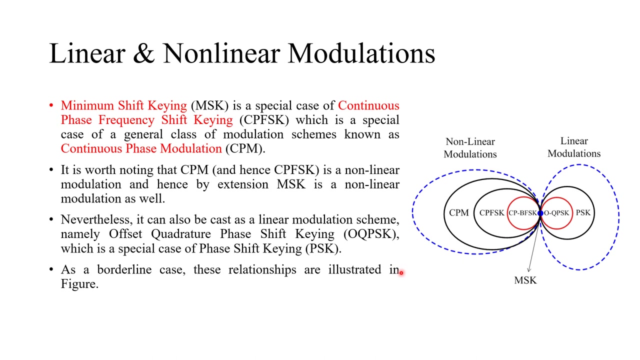 So, as I mentioned earlier, this particular module can not be entered in the next cycle, which means control is needed over the other two modes, Which means that the techniques selected earlier are significantly different to each other. You may notice that in many modules of constant modulation, the steps are indeed the same as the previous modules. 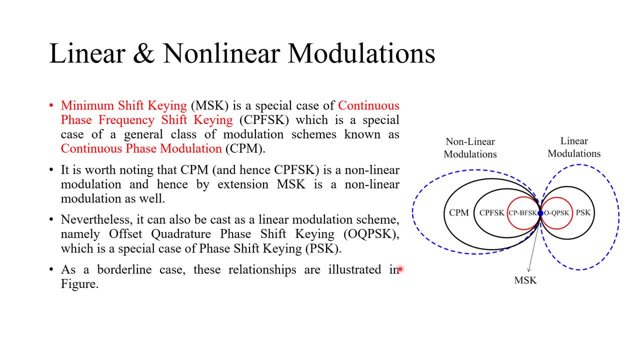 Now let's just a step back and let's have a comparison of the two modules. First of all we check the frequency range of the modules. But linear modulations will show a constant or a specific state of carrier signal throughout the symbol period, ie if PSK or QAM or QPSK, all these kinds of modulations will have a. 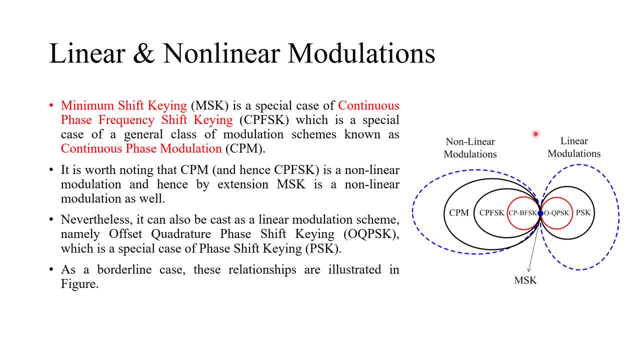 specific state of the carrier to represent a symbol, while in the non-linear modulation schemes the state of this carrier signal will reach a constant state, but it will be gradually reaching to that state so that it is not totally constant throughout the symbol period. Such systems are termed to be non-linear modulation. 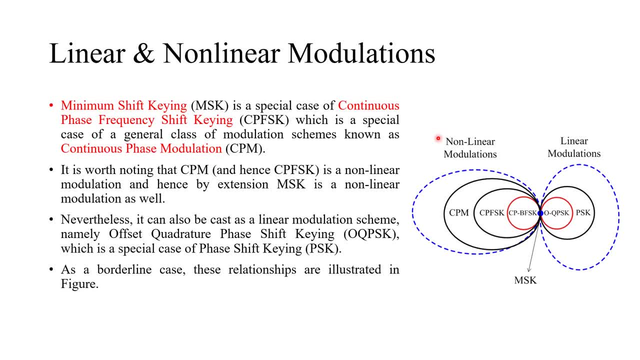 So in this continuous phase modulation is a broader classification in which continuous phase frequency shift keying is a special case and minimum shift keying is special case which comes inside the continuous phase frequency shift key. Generally, the minimum shift keying is considered to be a part of a non-linear modulation. 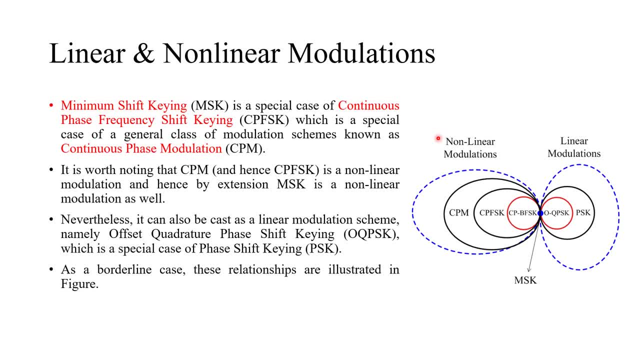 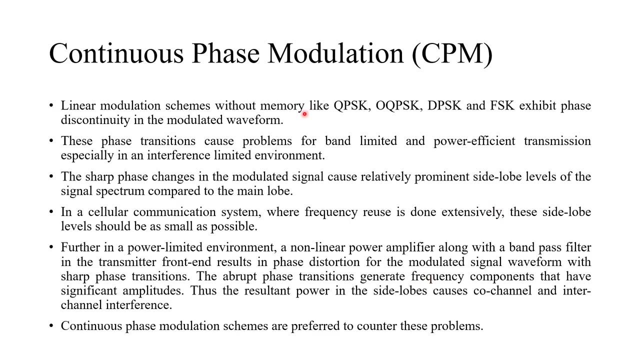 So moving on the non-linear modulations. but it also exhibits the properties of offset QPSK, which comes in linear modulation. So MSK is a borderline case which we can understand from the diagram. The linear modulation schemes like PSK and FSK, exhibits phase discontinuity in the modulated. 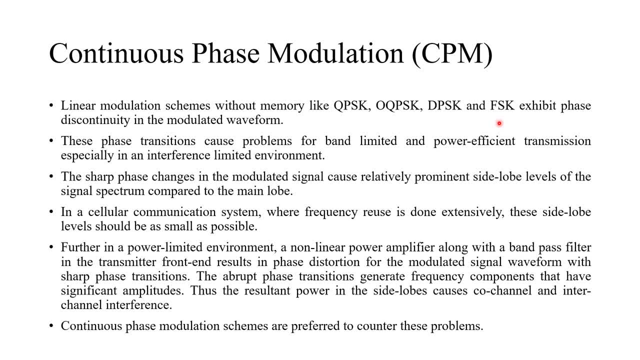 waveform- That is, the phase of the signal- keeps changing from one state to another. according to the input signal, That means the phase is not continuous. So such a sudden transitions in the phase will create high frequency components and unmounted frequency components in the 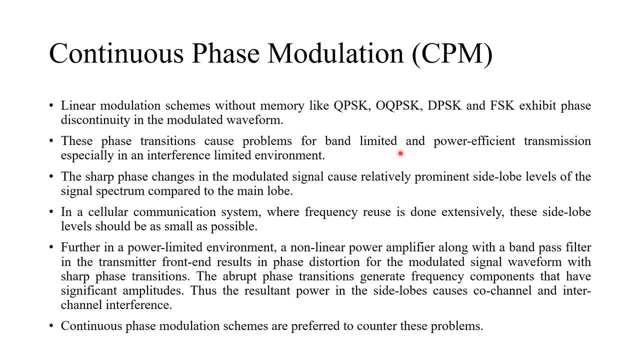 output spectrum which may cause problems of interference in the nearby channels and also will reduce the power in the same channel. So such phase transitions will cause additional frequency components which are a problem to the total system where the frequency band is continuously irregular. However, since PSK has high frequency components in the output spectrum, the PMT Joey is Montenegro. 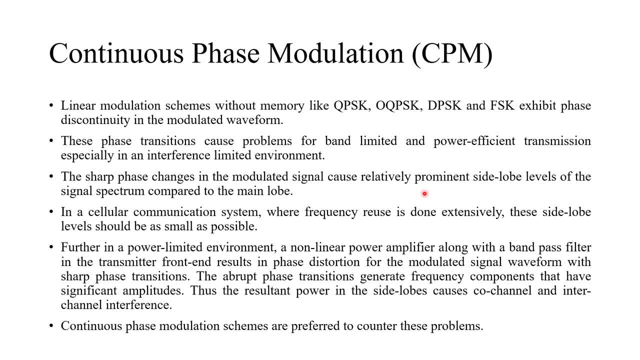 bullet strength will not be able to reduce the cooking helmet voltage. trabajar a hosted on The about 300 feet out 32 o about operation. So such non-linear amplifiers and filters may also produce additional frequency components due to the sudden phase transitions. So in order to avoid such additional frequency, 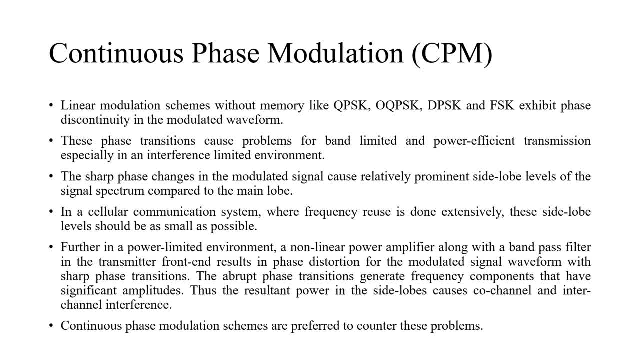 components. due to the phase transition, continuous phase modulation schemes are preferred. In continuous phase modulation schemes there is no sudden or no abrupt change in phase. The phase change will be gradual from one state to another, So the interference effects will be minimal. 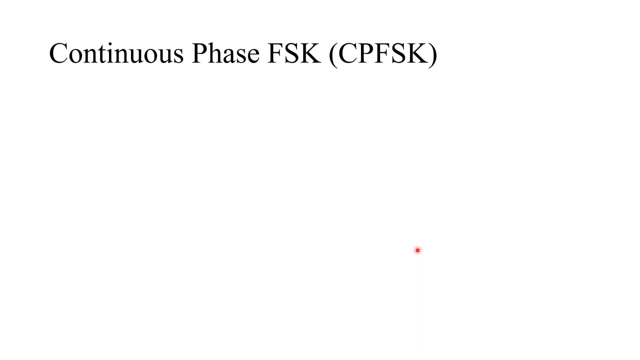 Now let us take a look at the normal FSK system and continuous phase FSK system. In the normal FSK we have a, as we all know, there will be two oscillators which generate two different frequencies, and those two frequencies will be switched bit according to the input bits, So there will be phase. 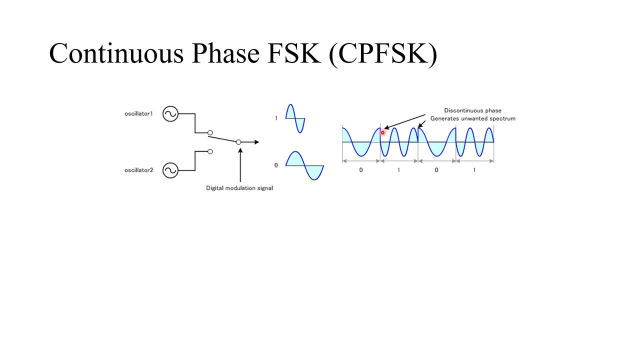 transitions when the bit changes, and these transitions are sudden from one state to another, and these sudden transitions will generate unwanted frequency components in the spectrum. So if It is a continuous phase frequency shift keying, instead of switching between two frequencies we can use a voltage controlled oscillator. 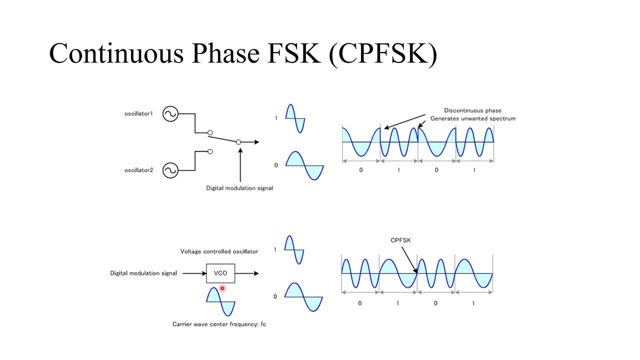 which will generate frequencies according to input voltage and as the input to the VCO, the digital modulation signal is provided. So when the input signal is high, the VCO will generate a high frequency signal, And when the input signal is lower than zero, 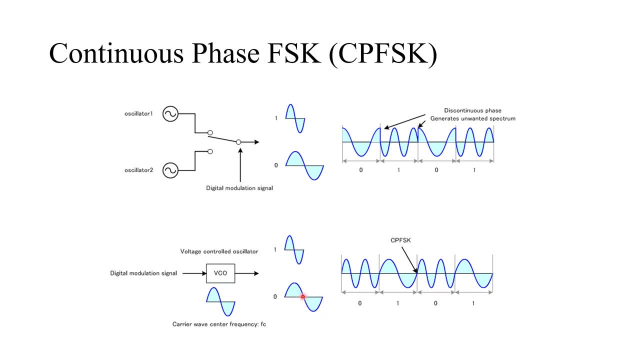 grow, then VCO will generate a low frequency signal and the change from the high frequency to low frequency and low frequency to high frequency will be continuous. There will not be any transition between the phases. It is continuous, as you can see. So this is the 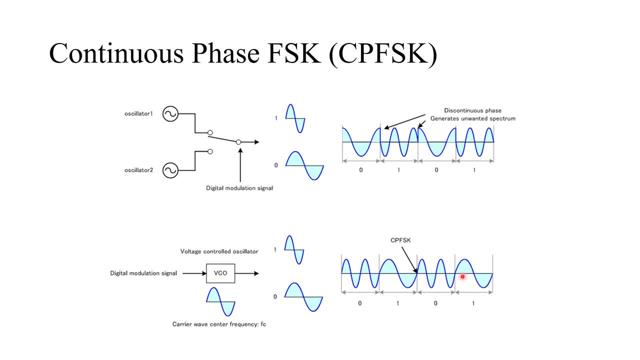 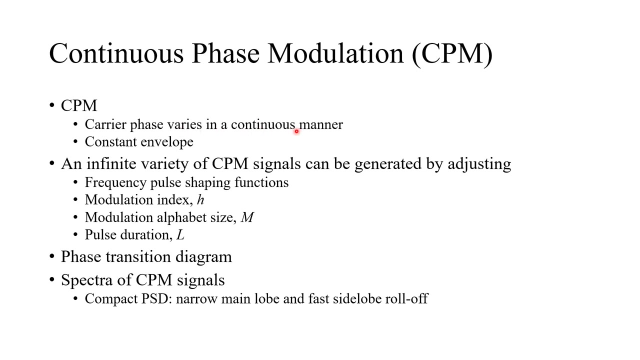 advantage of continuous phase frequency shift keying. This continuous phase frequency shift keying comes under the classification of continuous phase modulations. In continuous phase modulation, the carrier phase varies in a continuous manner and the envelope of the modulated output signal is constant. A large variety of continuous phase. 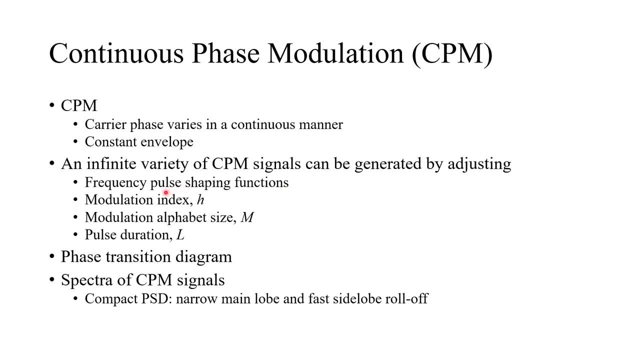 modulation schemes can be developed or generated by changing the pulse shaping functions: modulation index, modulation alphabet size and pulse duration. If we inspect the phase transition diagram of schemes like PSK and FSK, the phase change is up to 180 degrees, where in the case of CPM, the phase transition is smooth and minimum. 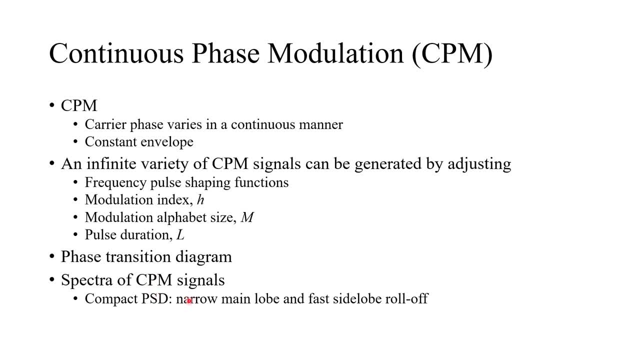 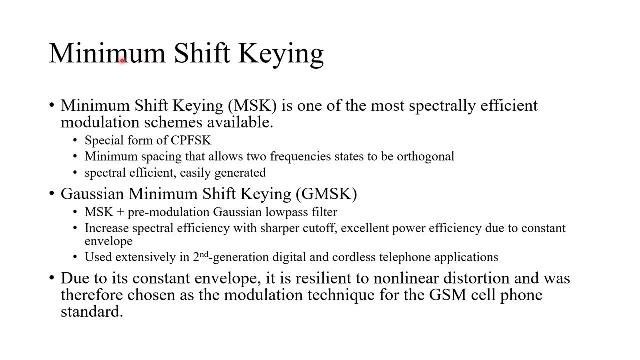 If we check the power spectral density of the CPM signals, the power is concentrated onto the main block. Minimum shift keying, or MSK, is a special form of continuous phase modulation. MSK is one of the most spectrally efficient modulation schemes available. It 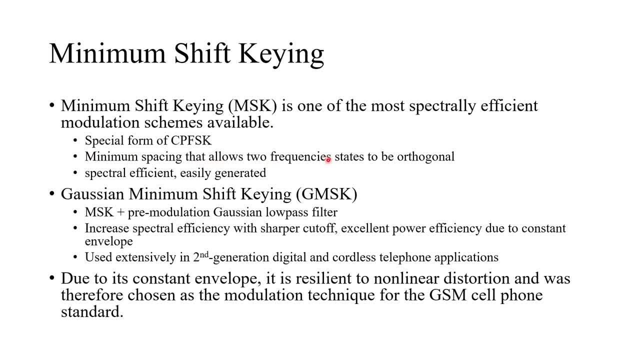 is allotted with a minimum spacing that allows two frequencies to be orthogonal, It can be easily generated. An advanced version of MSK is Gaussian MSK or GMSK, which is used in our GSM cell phone communications. In GMSK, a Gaussian low-pass filter is added in the 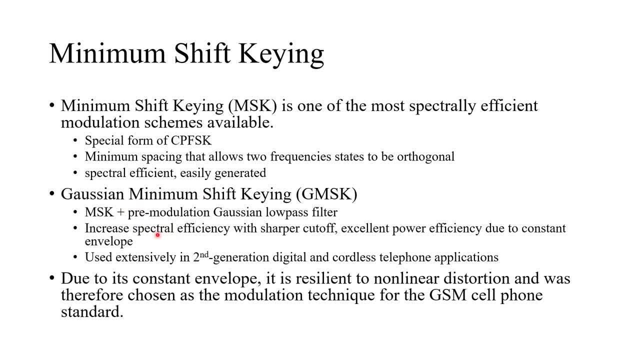 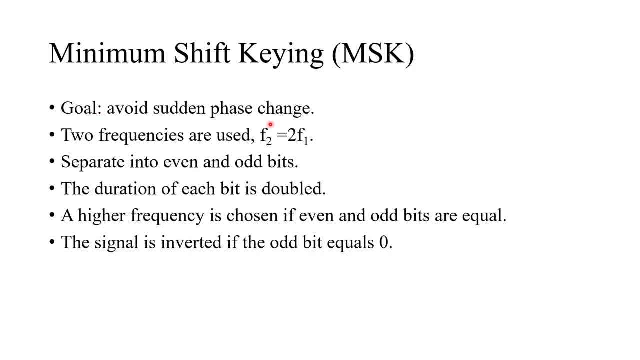 pre-modulation stage to increase the spectral efficiency of the system further. In MSK our aim is to avoid the sudden phase change, as this is a special case of continuous phase frequency shift keying. This is similar to frequency shift keying. We have two frequencies. 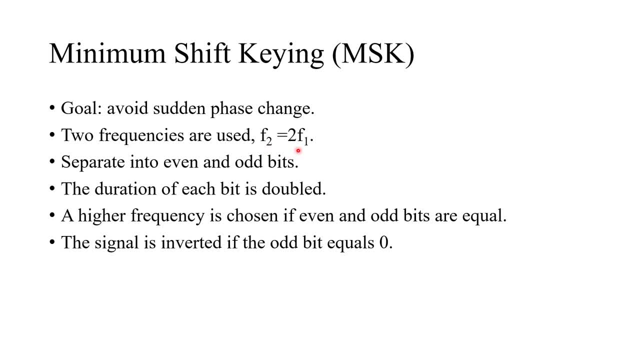 F1 and F2, and one frequency is twice the other frequency, and the incoming bit stream is divided into even and odd bits, And to keep the bit rate constant, the duration of each bit is doubled. The modulation is done in such a way that a high frequency is chosen. 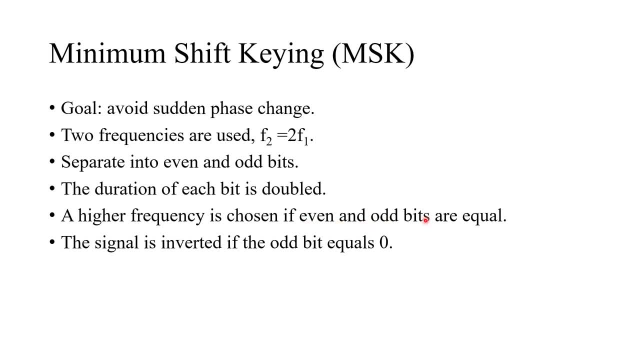 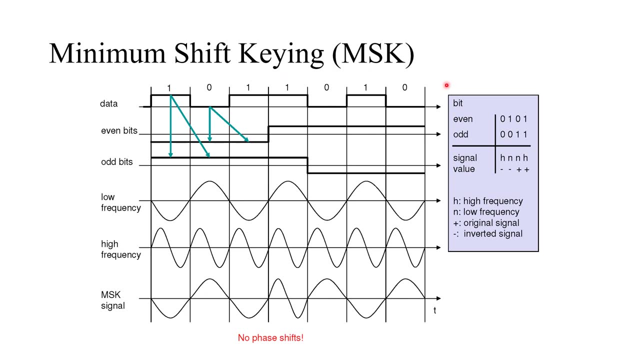 if the even bit and odd bits are equal at a time and the signal is inverted if the odd bit is zero. We shall see how this operates. Let us consider a sample bit stream of 10110,. here this is the input data stream and it is divided into even bits and odd bits. Here 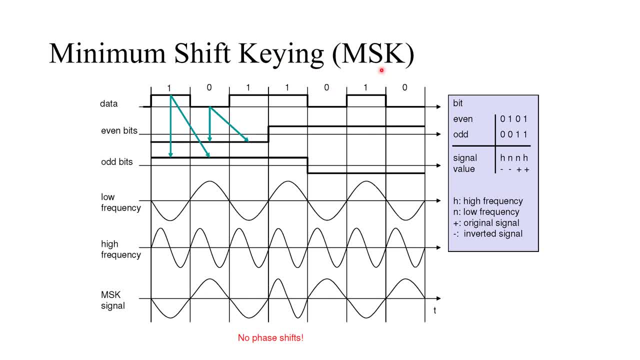 the odd bits are 1,, 1,, 0, 0, and the even bits are 0,, 1,, 1.. Here, first we will select the odd bit. here this 1 is the odd bit. the first odd bit is 1, and its time duration. 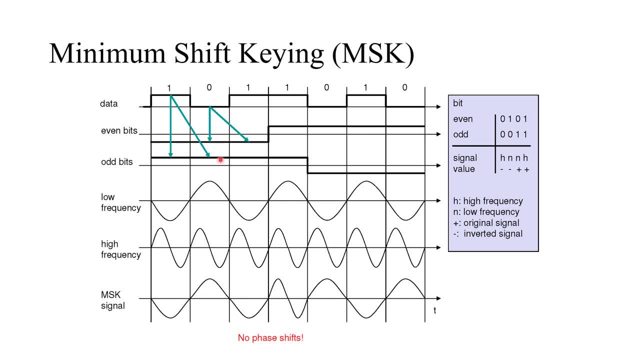 is doubled, So 1 is the odd bit. the first odd bit is 1, and its time duration is doubled, So 1 is continued to the second bit, duration, and then the next odd bit is again 1,, so it. 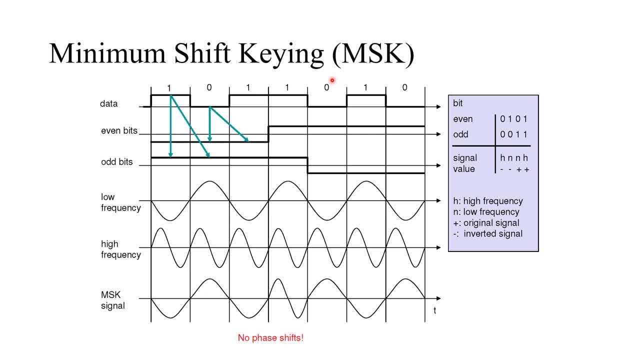 is continued to the next bit- duration- and then the third odd bit is 0,. it is doubled. and then the next odd bit also is 0, and it is continuous as such. So now let us consider the even bits here. the first even bit is 0, its duration is doubled. 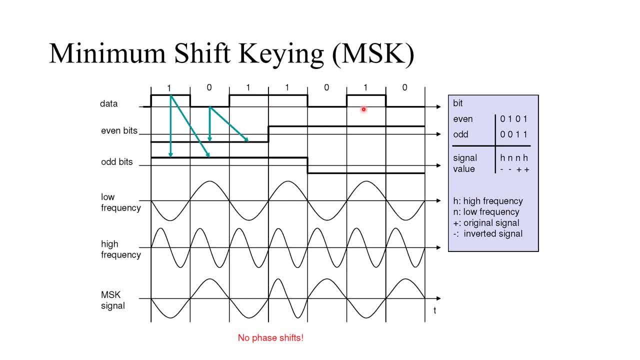 the next even bit is 1, its duration is doubled. next even bit is 1, its duration is doubled. And this is the reference table for the operation of this MSK scheme. Here the high frequency is denoted with H, low frequency is denoted with the letter N and the original signal. 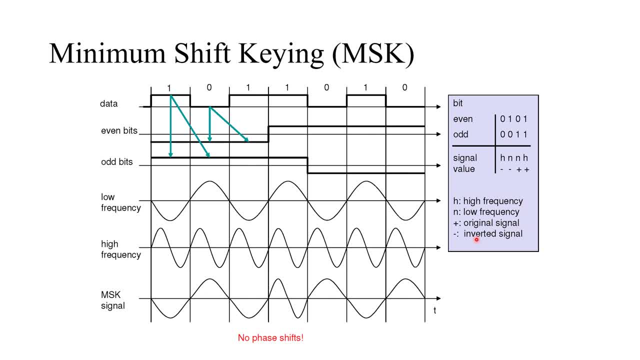 is denoted with positive or plus, and the negative signal, or inverted signal, is denoted with minus or negative. OK, Ok, frequencies. one is a low frequency and one is a high frequency, which is twice the low frequency. now let's see how the output is generated, bit by bit. so at the first bit condition: 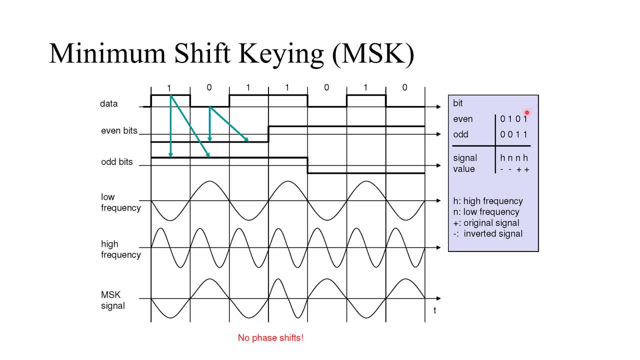 the even bit is 0 and the odd bit is 1 for. so here for a 0: 1 condition, the output should be low frequency in its original form. so we will transmit the low frequency signal with in its original form. in the next bit period, again it is 0, 1, so we will transmit the low frequency. 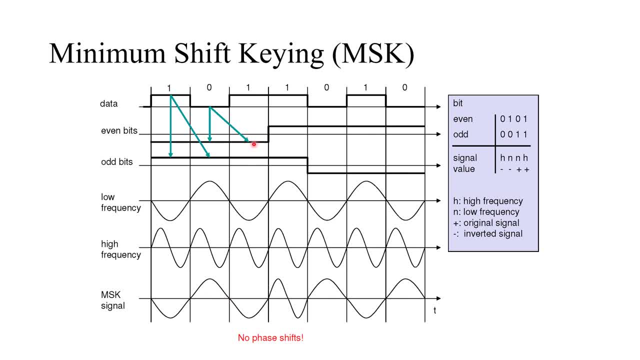 in original form. in the third bit period also it is 0, 1, so low frequency in original form. for in the fourth bit time the state is changing. here we have 1, 1, so for 1, 1 condition we have to transmit the high frequency in its original form. so instead of this low frequency we will transmit 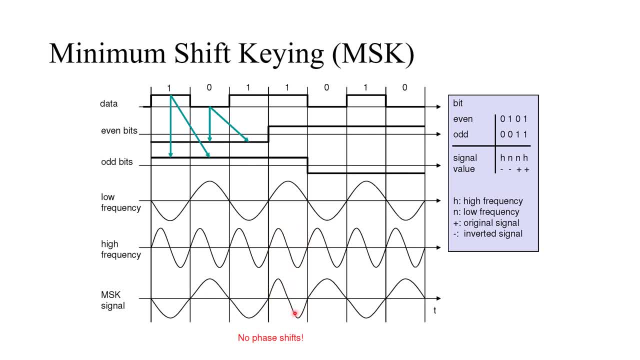 this high frequency in its original form. the next state is 1: 0- 1: 0. we have to transmit low frequency, but inverted. so in the case of 1: 0, we will transmit this low frequency, but inverted. again, it's 1: 0- low frequency inverted. 1: 0- this low frequency inverted. so in effect, 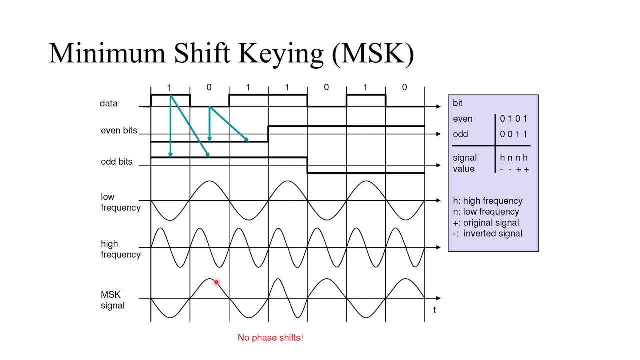 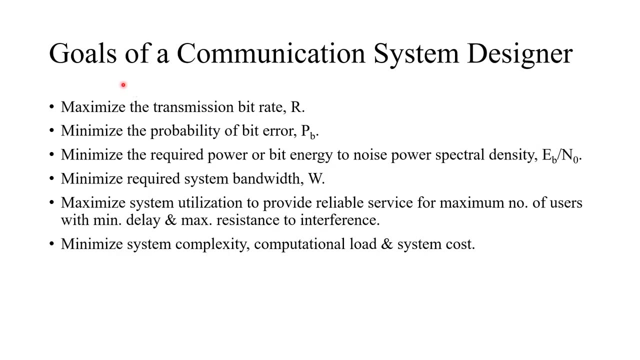 an msk signal is generated and, as you can see, there is no phase shift. all the phase changes are gradual. this is the scheme for the generation of msg. the goals of a communication system designer is to maximize the transmission bit rate, or the throughput, and to minimize the probability of error. he 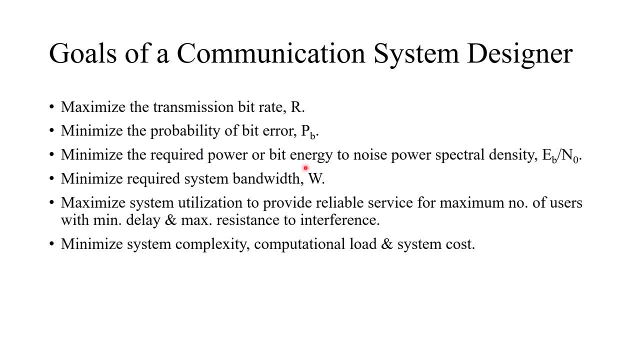 also aims to minimize the required power or bit energy, to maintain a satisfactory signal to noise ratio and to minimize the rester system bandwidth. he also has to maximize the utilization of resources available for the service of maximum number of users, with minimum delay and minimum interference. he also has to 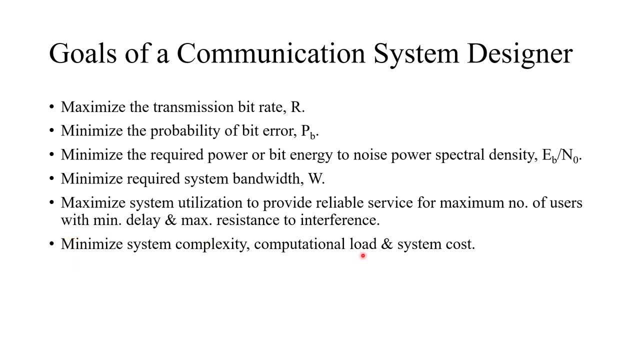 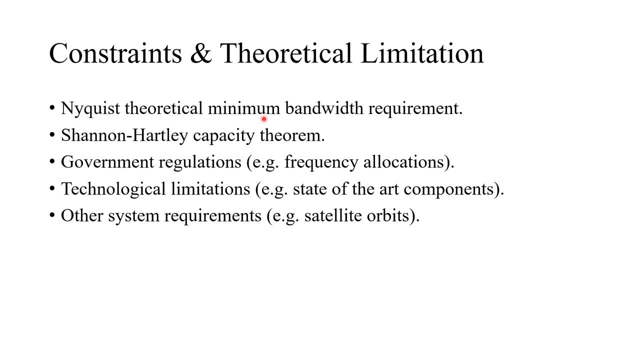 minimize the system complexity, computational load and, of course, the system cost. the constraints and theoretical limitations in designing such communication systems are mainly the next minimum bandwidth requirement, which states the need for sampling a signal at minimum twice its frequency. and then there is the Shannon-Hartley capacity theorem, which describes the 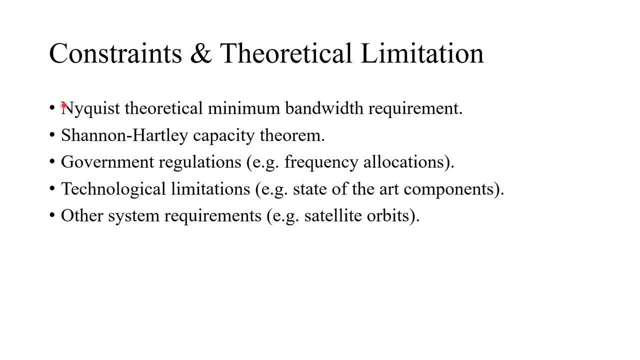 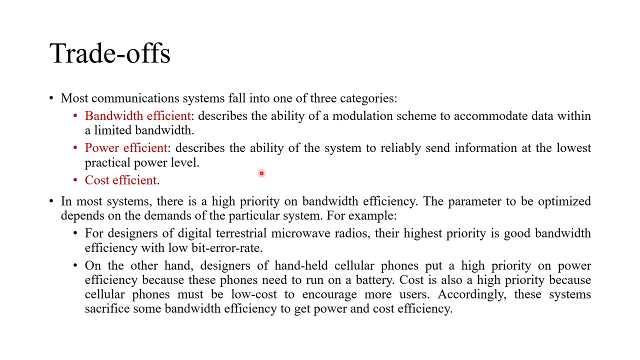 maximum amount of data that can be accommodated in a certain frequency. then there are government regulations in using certain frequency bands. then there is technological limitations in the availability of the state-of-the-art components. then there are other system requirements too. send information at the lowest practical power levels. in most systems there is a. 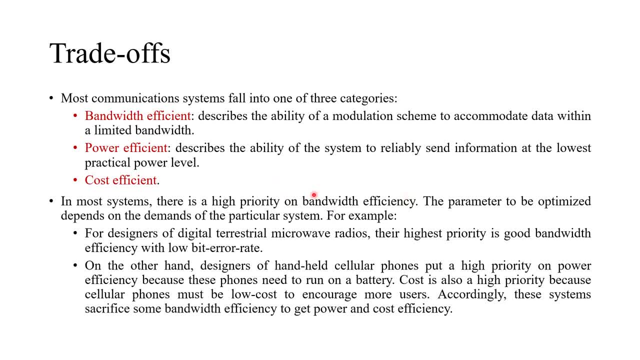 high priority on the bandwidth efficiency, because bandwidth is the most costly one. the parameter to be optimized depends on the demands of the particular system. for example, if it is a digital terrestrial microwave radio, their highest priority will be a good bandwidth efficiency and low bit rate. they don't have to worry about the power, because it's not a